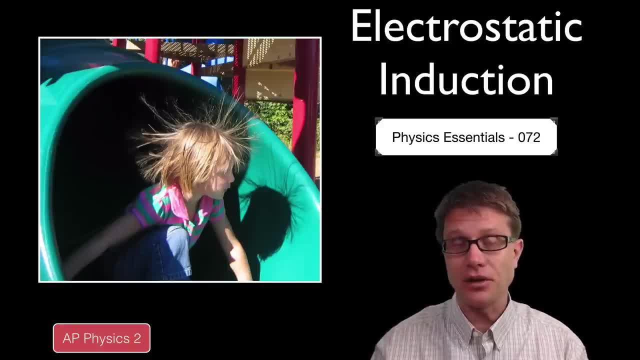 the slide friction of their hair. on the slide actually pulled electrons off, And so now all their hair have positive charges, And so that induction of the hair itself is pushing on all the other positive hairs, And so we get this crazy looking hair, And a good way. 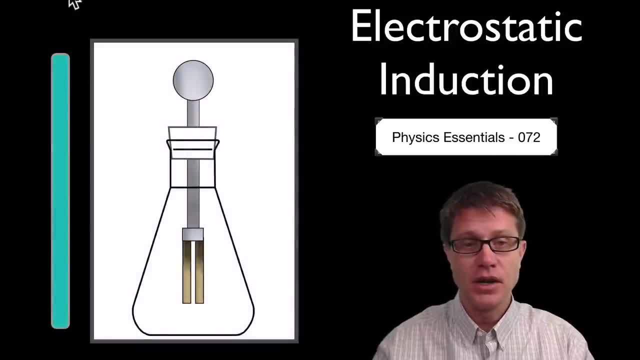 to study this in the science lab is to use something called an electroscope, And so what we have is a metal ball at the top, connected to a metal rod that goes through the middle, And then we have metal leaves on the bottom, And so these are all insulated from the surroundings. 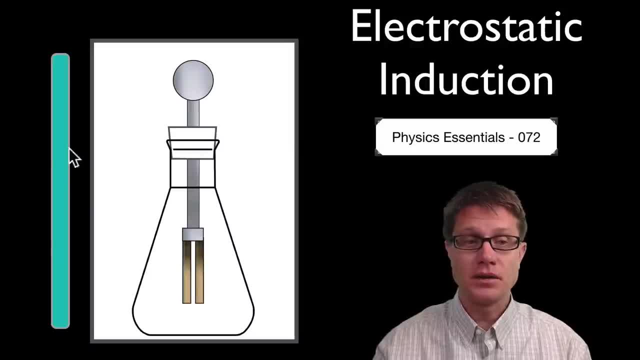 because we have a rubber stopper that goes right around here. And so what we are going to do is we are going to charge up a glass rod And so we are going to put this metal going to charge up a rod like that, And so what you are doing is actually pulling electrons. 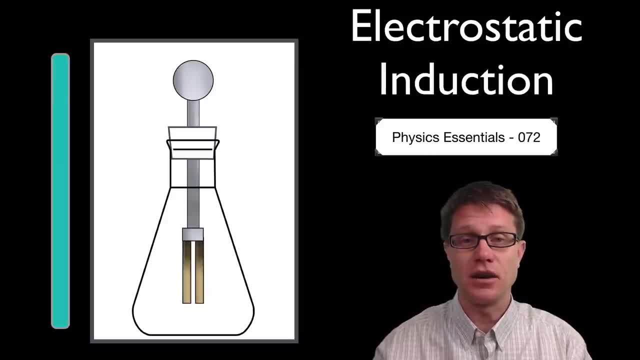 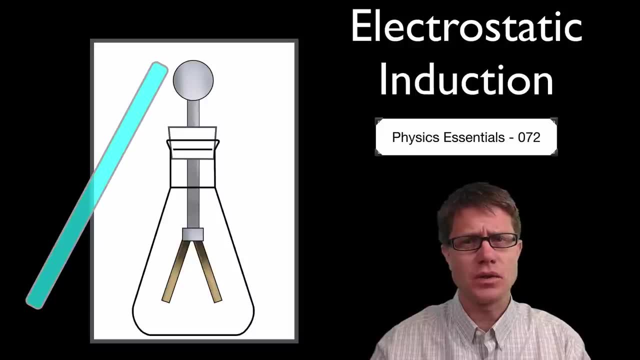 off of it And now we have a positive rod. It is just like the hair of the child, And so as you pull it close to the electroscope, what is going on is induction here, So it is impacting the charges within the electroscope. Watch what happens as we pull it away. The 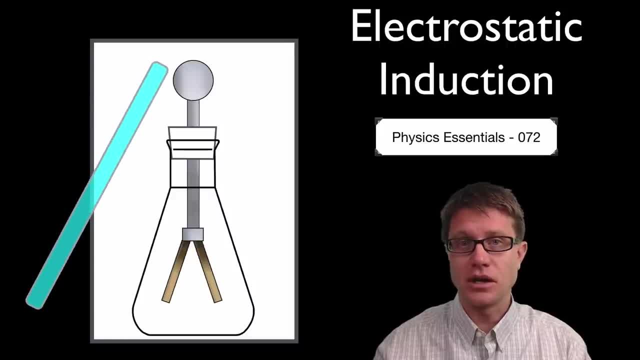 leaves go back to where they were As we put it closer. there is induction going on. As we pull it away. they go back. What happens if we actually touch it? So if I touch that now, conduction takes place. So we are actually transferring charges And watch what happens. 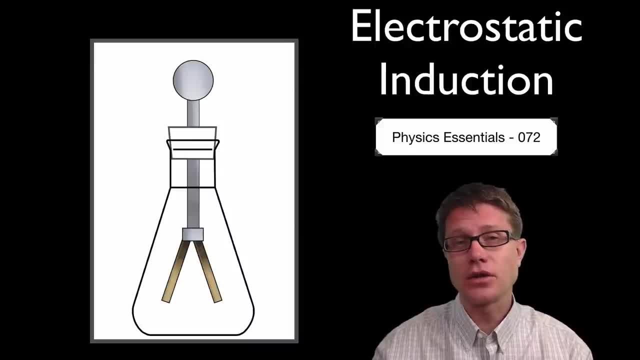 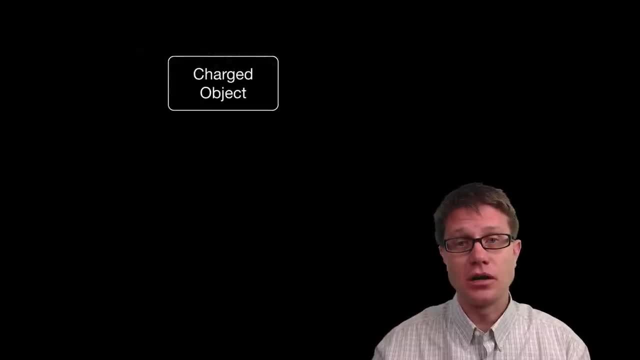 as I pull it away, Those leaves are going to be held apart. So to understand what is going on at the charge level, you really have to understand what electrostatic induction is, And so a charged object can be charged through friction, like rubbing your hair on. 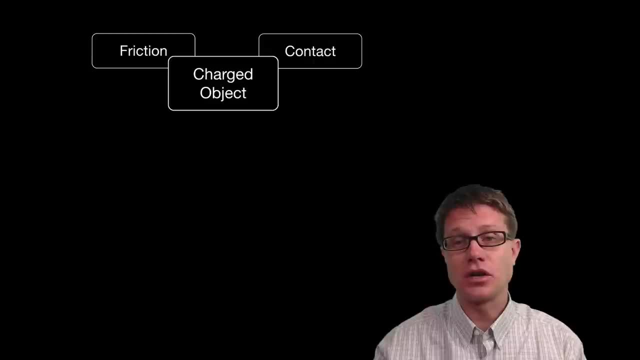 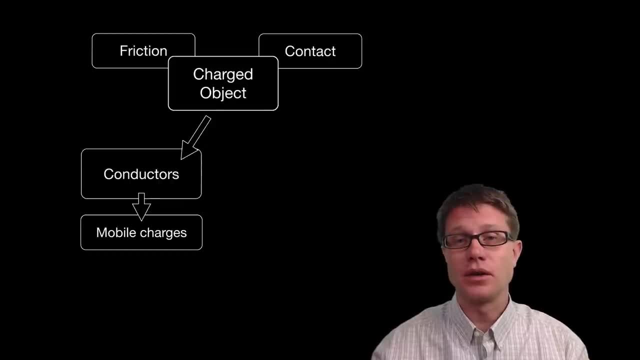 can move around, and that charge is going to start to dissipate or at least move within the object itself. If it is an insulator, all of those charges or those electrons are fixed, And so we can add charges to one part of it, And it does not mean the rest of it has to. 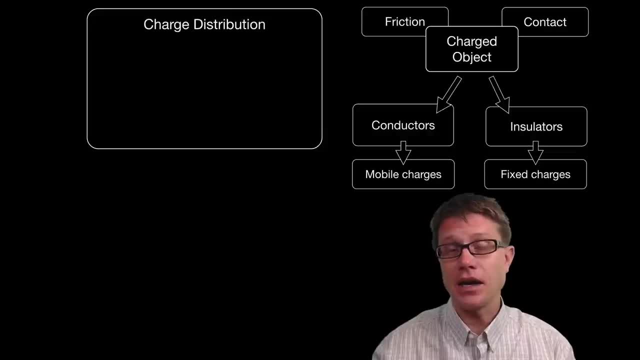 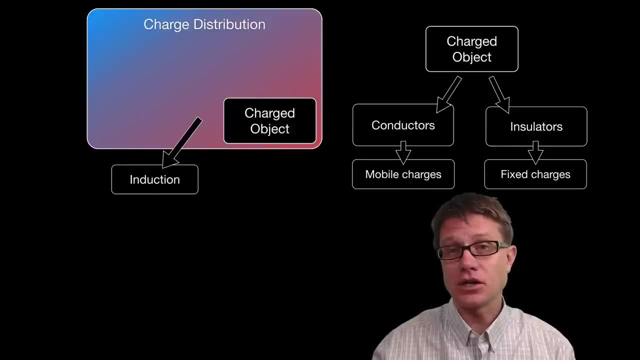 stay charged. But if we take a charged object and we add it to a system, we are going to change the distribution of the charges within that system, And so if we do induction, it means we are going to move it next to another object, but we are not physically touching. 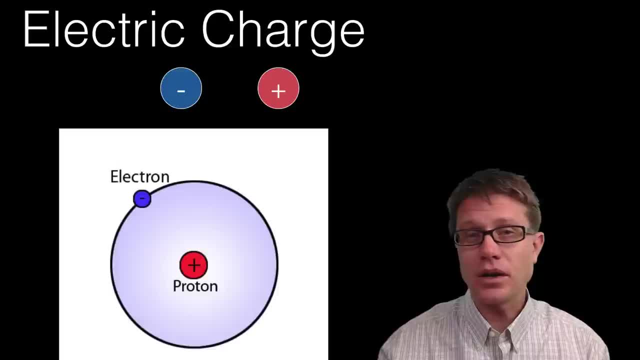 it. And if we are doing conduction, then we are going to physically move it, And so that does not mean we are going to physically touch it. And so what are these charges? Remember, it is going to be the electrons and the protons in the atoms that make up the material itself. 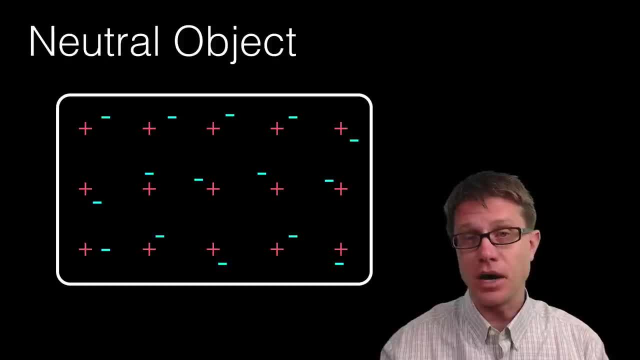 And so if we have a neutral object, that means we are going to have an equal number of positive and negative charges. They are going to balance out and there is going to be no net charge. Now, what does a charged object look like? Well, in this case we have way more negative. 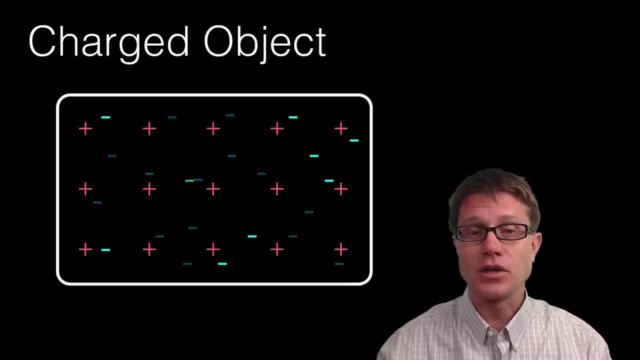 charges, and so this is going to be a negatively charged object. What is it going to look like if we pull those electrons away? Now we are going to have a positively charged object, But remember, the protons are going to stay where they are. It is always the electrons. 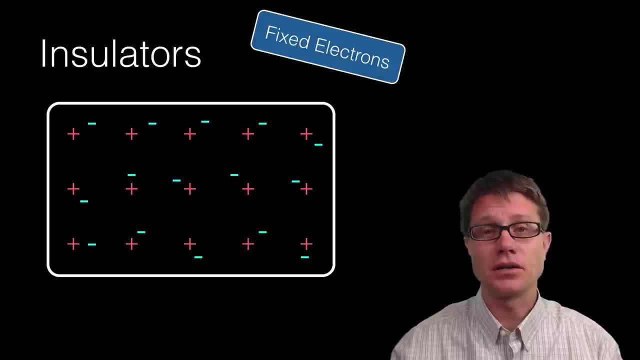 that are moving. Now, how is an insulator different from a conductor? Well, in an insulator, like in glass or in plastic, all those electrons are fixed, And so they can move a little bit, but they are always going to be stuck to that proton of the atom of which they are a part. 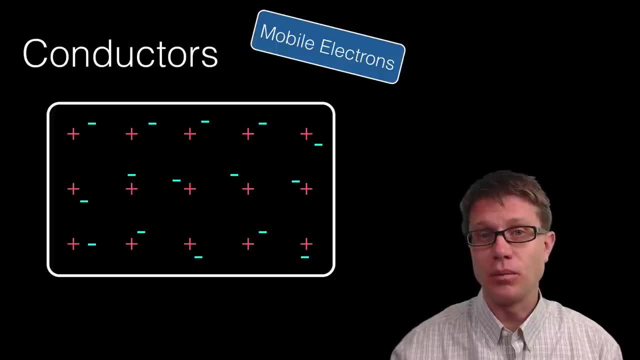 Now, how is that different in a conductor? In a conductor, remember, those electrons are mobile, It is a sea of electrons, And so those electrons can move around. And so when we have a conductor and a charged insulator, they are going to behave in different ways, And 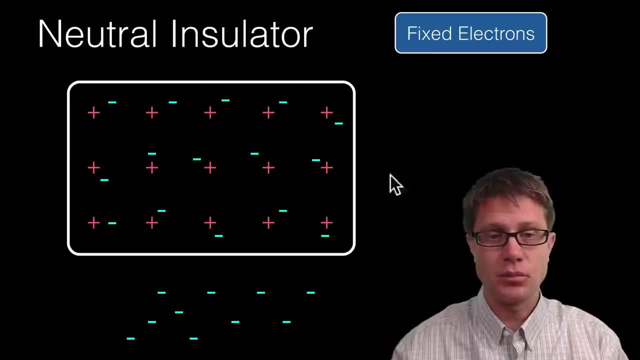 so if we have a neutral insulator like this, So this is a neutral insulator up here, So we have an equal number of positive and negative charges. But what I am going to do is I am going to add some negative charges to it. So when I add those negative charges, like 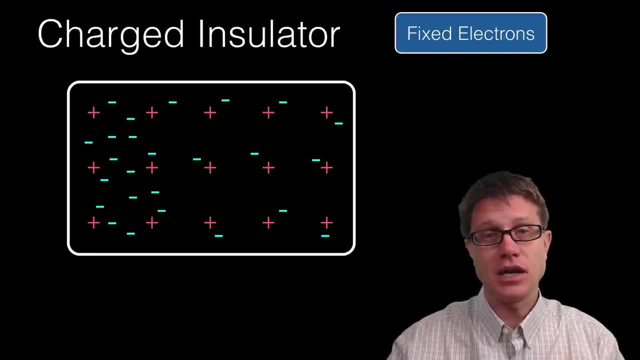 that those electrons are fixed in their position. They cannot dance from atom to atom. And so what are we going to have now? A charged insulator, where the left side in this diagram is going to have a negative charge And the right side is going to have a positive charge And the 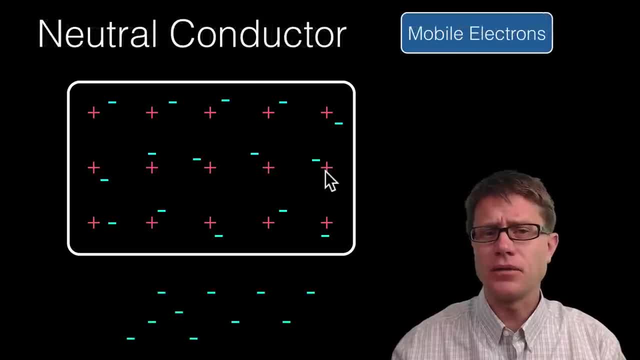 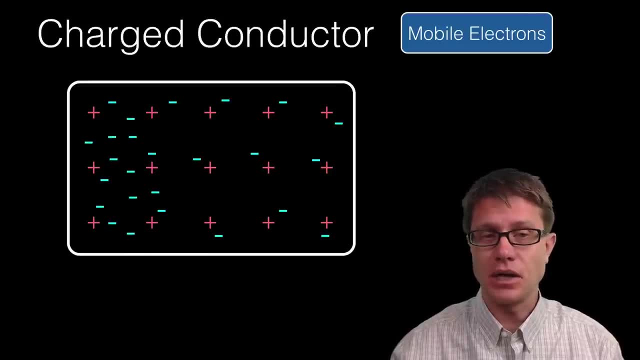 right side is going to have a neutral charge. Now, how is that different than a conductor? Well, same thing. We are going to start with a neutral conductor now And I am going to add a bunch of charges to it. Same location, But what happens with these electrons, is they? 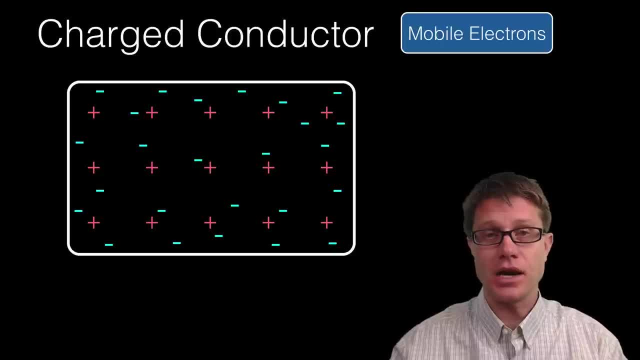 can move. They hate being around other electrons and so they are going to spread out And that charge is going to start to be on the outside of that conductor. So remember, in a conductor, if we are ever dealing with metal, those electrons are moving, But if we are dealing with an 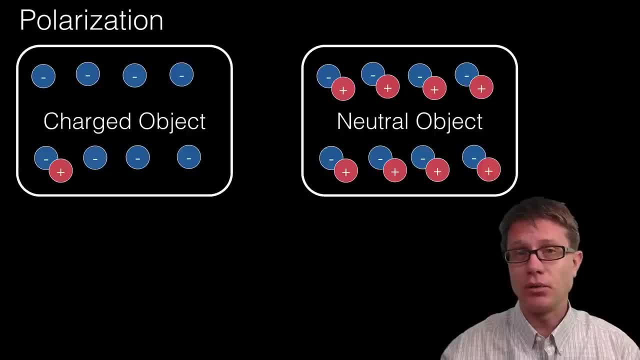 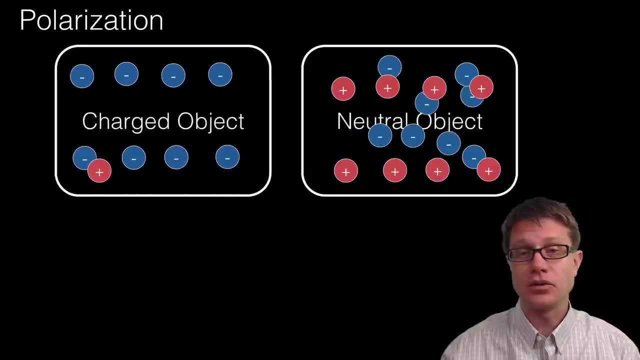 insulator. they are going to remain fixed in position. And so what is polarization? It is when I can take a charged object like this one, where we have a lot of electrons, and as I move it near a neutral object, what is going on? You can see those electrons are. 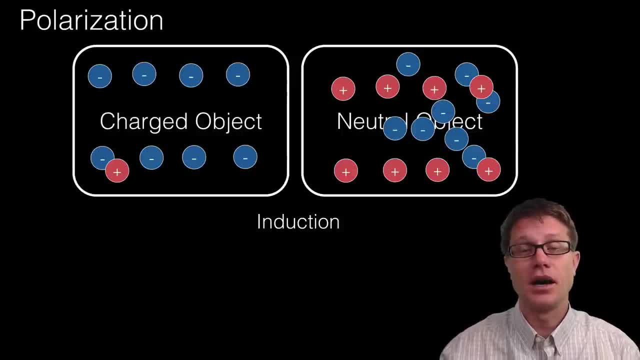 moving. So we know right away that this is going to be a conductor, since the electrons are moving. But since it is not touching, now we have electrostatic induction taking place. What happens if I actually touch it? Now we have conduction. Those charges can actually. 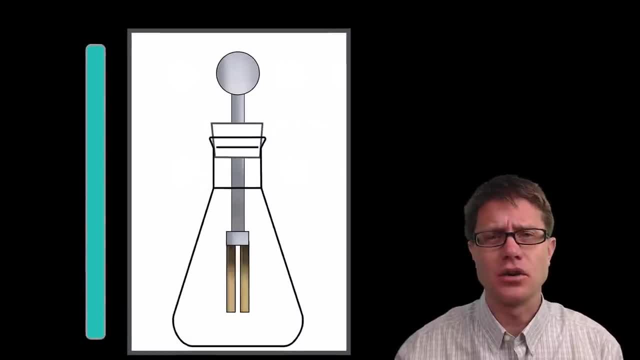 flow from one to another. So now let's go back to the electroscope and try to discover what is going on at the charge level. So again, I took a glass rod and then I charge it, And so what I am really doing is pulling the electrons away, And as I move it close to that electroscope we can see that. 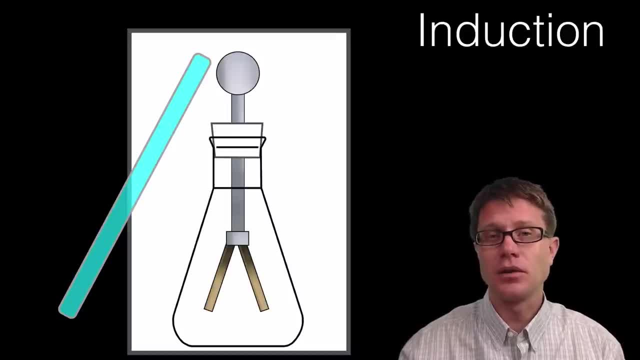 those leaves at the bottom. those metal leaves are moving apart And so let's kind of draw the charges out here. So this has a positive charge on our rod, So we have removed electrons from it. So why do we have a bunch of electrons up here? 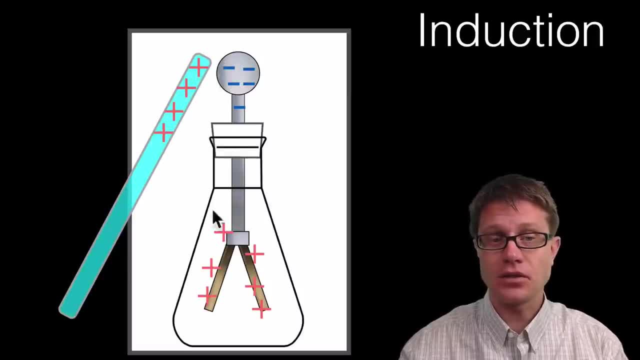 Because as we move the positive charges close to the conductor, the electrons in the whole conductor itself- remember, this whole thing- is connected. those electrons are moving up because they are attracted to the positive charges in the rod. What does that leave behind? It leaves behind all these positive charges. And since we have positive charges on this, 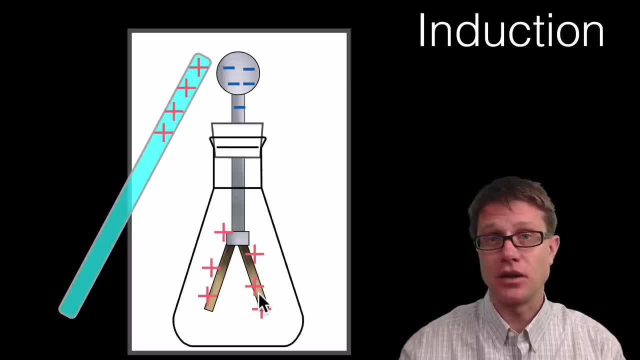 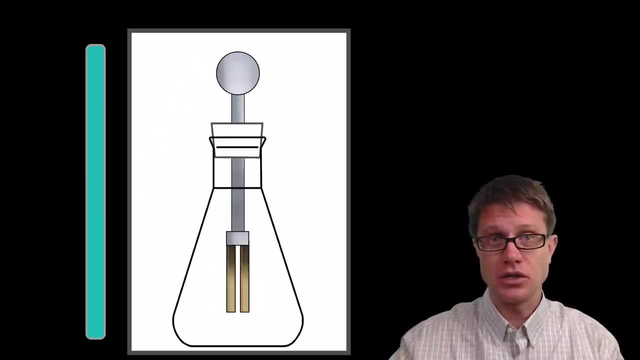 side, Positive charges on that side. They are pushing against each other, and that force is actually causing those metal leaves to move apart. If I move the rod away, it goes back to where it was. Those electrons are just going to dissipate. now we have a neutral electroscope. What happens, however, if I touch it? if there is conduction? 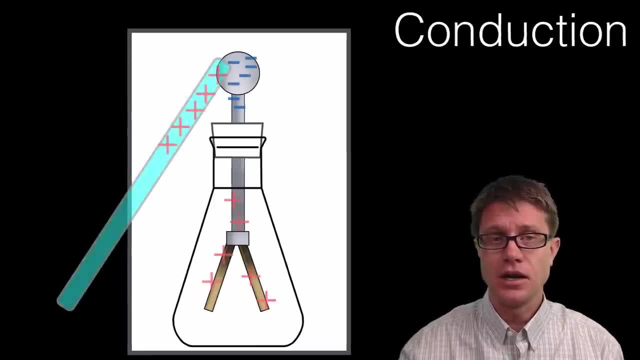 taking place. I pull it away and those leaves stay there again. what is going on? Well, we still have these positive charges up here. We have these electrons that moved up, So we have these negative charges over here. But since I am physically touching it there, 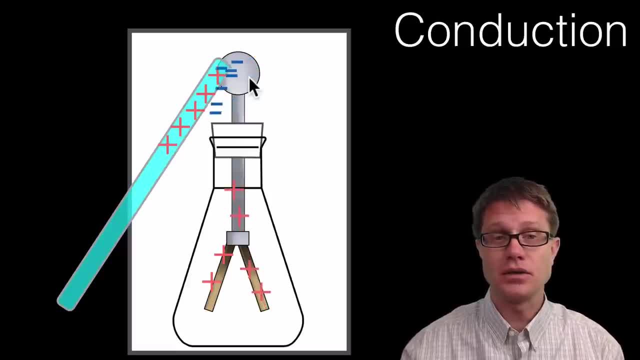 is now a pathway for those electrons to move, And what they are going to do is they are going to migrate over there. Now, this is going to be a neutral object over here, But what we have left behind are all these positive charges Since we pulled those electrons away. 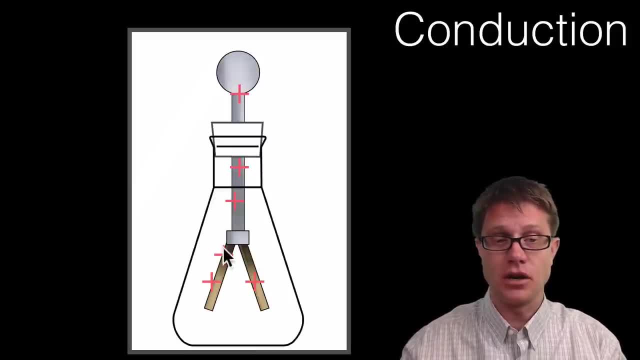 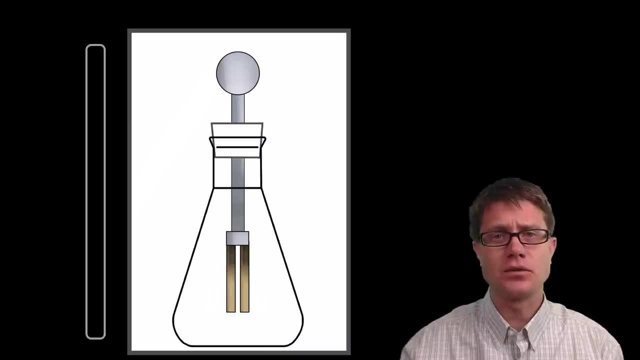 through conduction. now we are left with just the positive charges. All those positive charges are pushing on each other And then the leaves are going to separate. Now let's say we were to try, instead of a positive object, we were to try a negative object. So let's say we 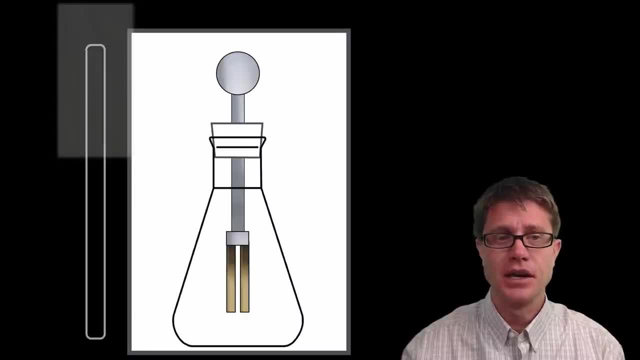 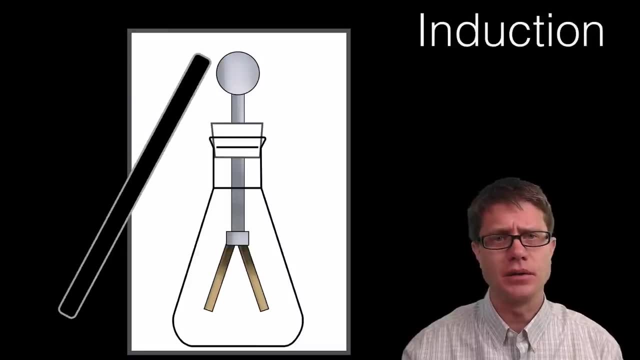 try a plastic. at this point We are rubbing the plastic. In this case, what we are doing is we are actually adding electrons to it. As I move it next to that electroscope, same thing happens. So what is going on there? Well, now we have the negative charges over here, So in the conductor of the electroscope. 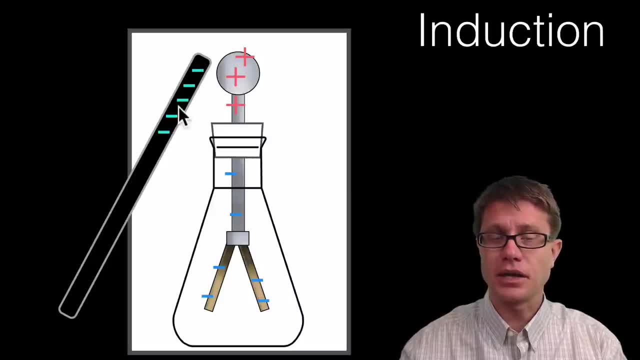 what happened to those electrons? Again, they are repelled by the electrons in this plastic rod And so they are moving down to the bottom, And since we now have a bunch of negative charges on either side, then it is pushing them away. What happens when we get conduction? 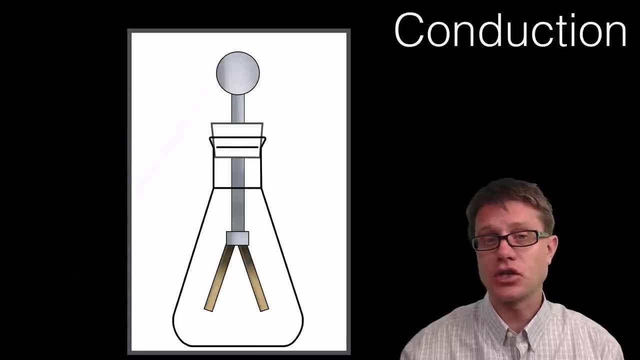 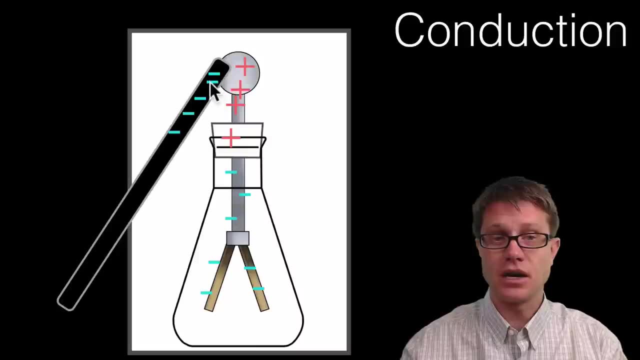 with a plastic rod. Again, if we look at it at the level of the charges- since this is negative charges right here- as we pull it closer all the negatives go down to the bottom, But these are not fixed. Once we touch it, these electrons can actually move through. 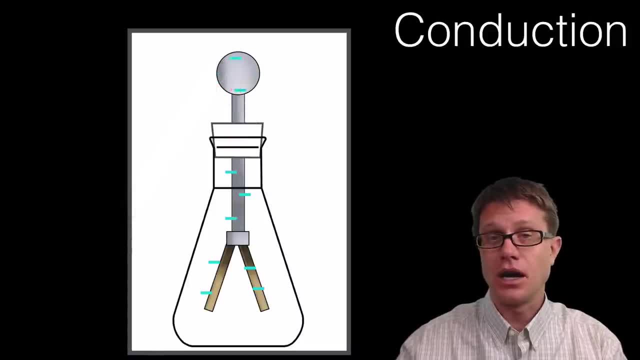 the conductor, And as they do that, we add a bunch of electrons to the conductor. It now has a negative charge And that is a permanent negative charge. It is going to stay that way until we can transfer those electrons somewhere else. So did you learn to make predictions? 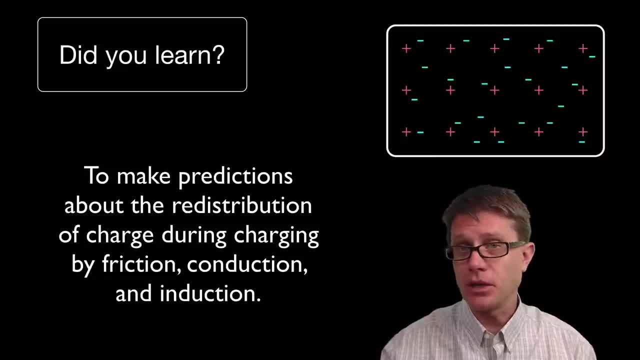 about the distribution of charge using friction. Again, when we are rubbing an object we can actually pull electrons off Or add electrons to it. Conduction: we are touching two objects so electrons can move, But induction: we are just moving where they are because they are not physically touching. 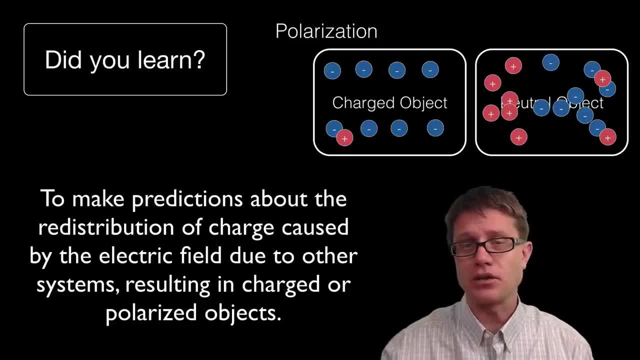 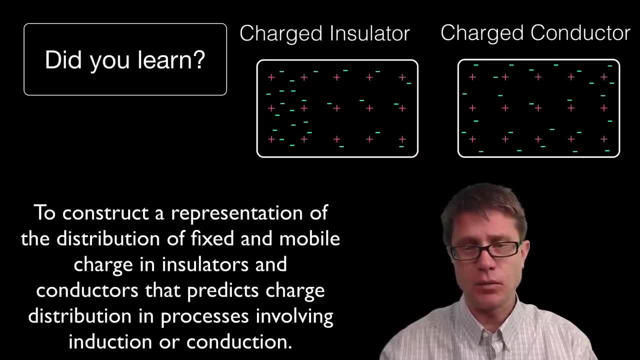 Could you make predictions about the distribution? when we are polarizing an object, Electrons again are moving. Could you construct a representation of how charges are going to be different in an insulator versus a conductor? Remember, in an insulator the charges are going to stay. 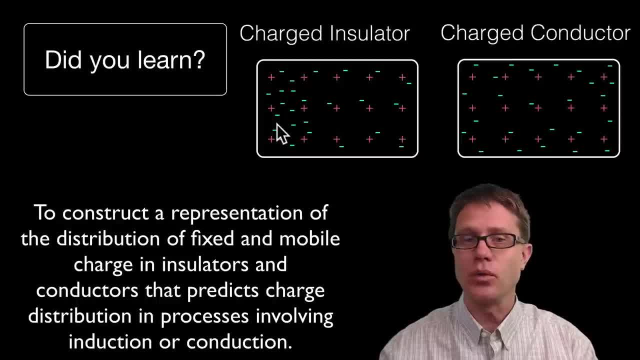 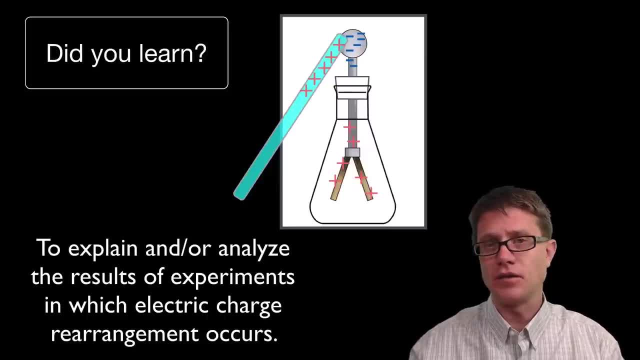 They are going to be fixed wherever you put them, But in a charged conductor they are going to move away from each other. And then, finally, could you explain the results of an microscope, for example, using charge and these ideas of induction and conduction? 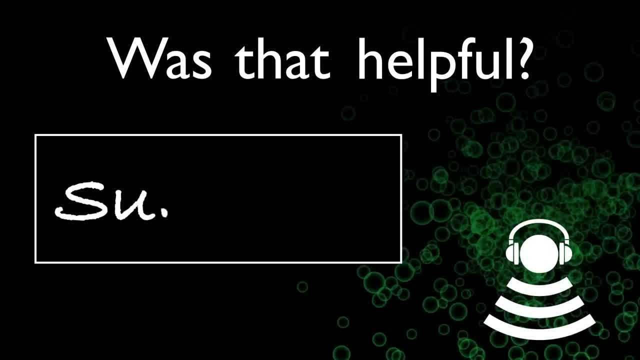 I hope so And I hope that was helpful.